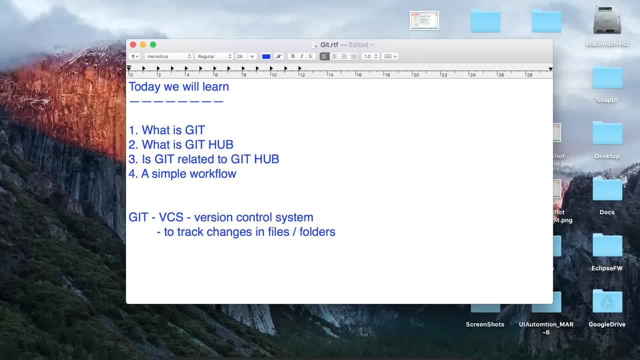 want to track the changes that we make to our source code or to our files or to our folders, And for that we use a version control system. And then we use a version control system to track the changes that we make to our source code. So in simple words we can say: to track. 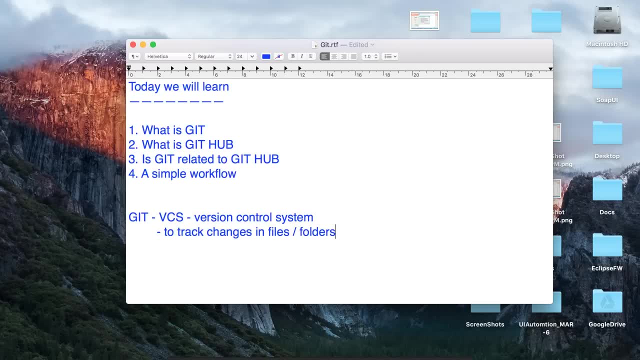 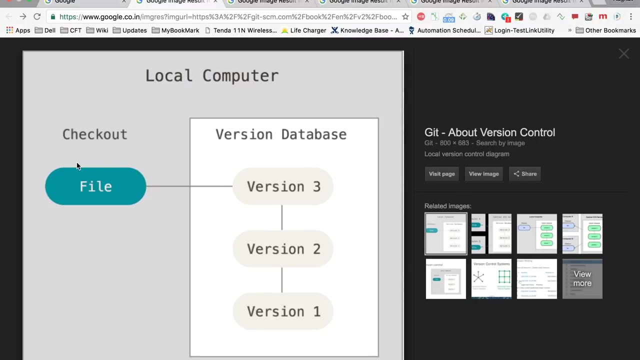 changes that we make to our source code, And then we use a version control system, And Git is a kind of version control system. The other reason we want to use Git will be to collaborate in teams. Okay, so let us again see this diagram. Here we are working on our 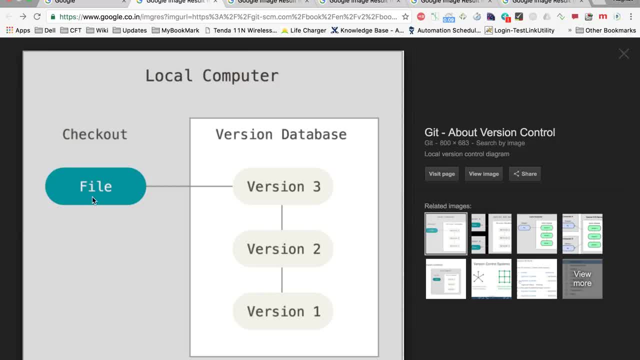 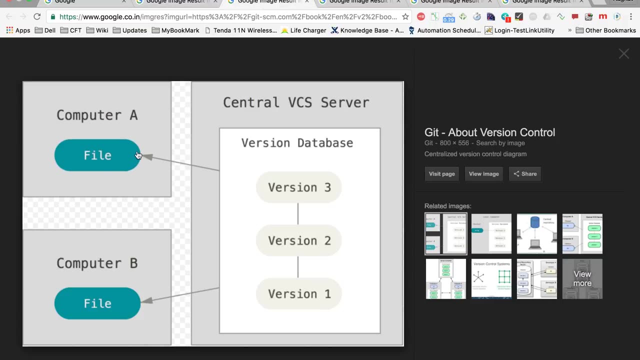 local system and we have a single file that only you are working on. In that case it makes very little sense to use a version control system Because you are the only person who is working on this particular file. But let us imagine when there are multiple people working on the same file. In that case, version control 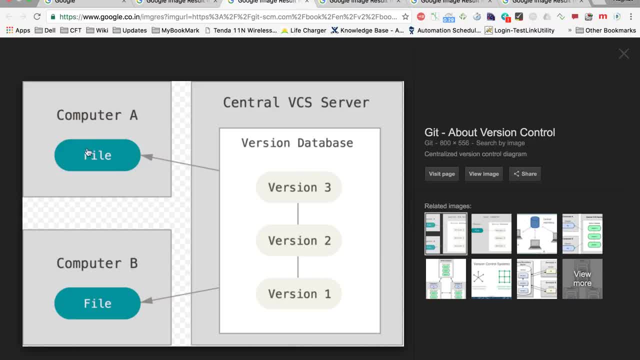 systems becomes very important because a person A checks out the file and he makes some changes, and a person B again checks out the same file and makes his changes. Now, in that case, we want to check all the changes made by Git. So let us say that we want to track all the 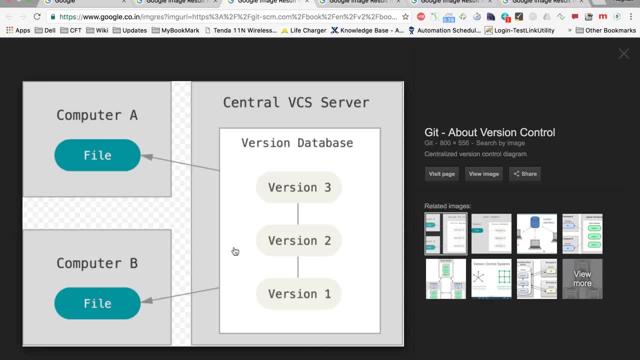 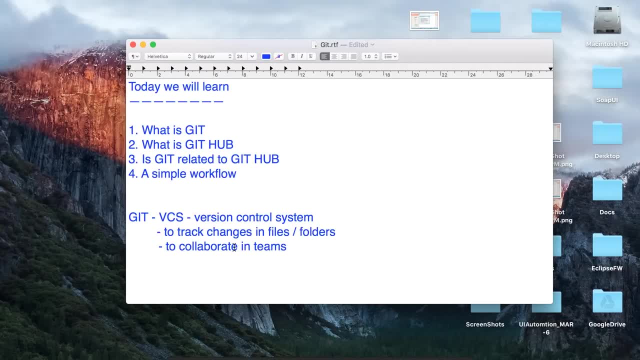 changes that we make to our source code And in that case we want to track all the changes made by all the people on that particular file. So in that case version control system becomes very important And that is why we use tools like Git to check the changes in. 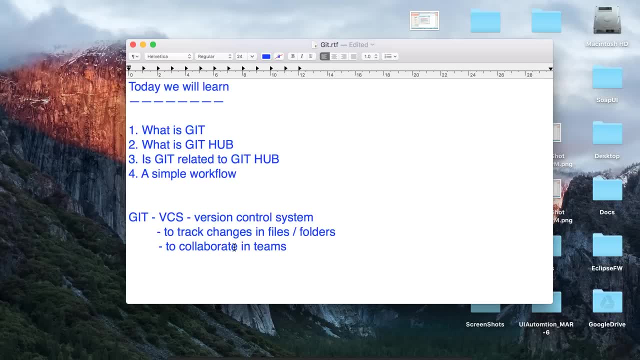 your code or in your files and folders. So this is what Git is and this is why Git is used. Now let us learn about version control system. We have two types of version control systems. One is centralized version control system, And then we have a centralized version. 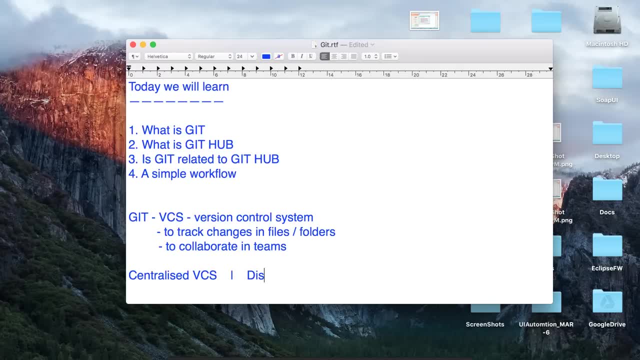 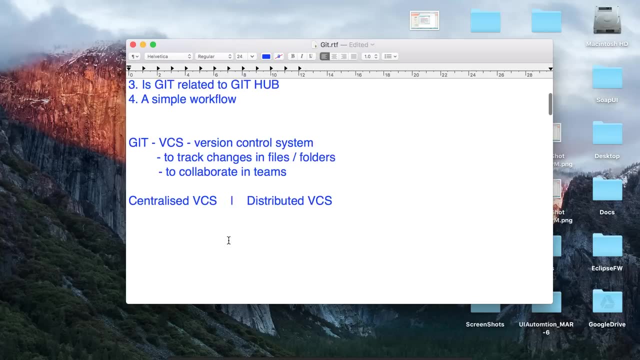 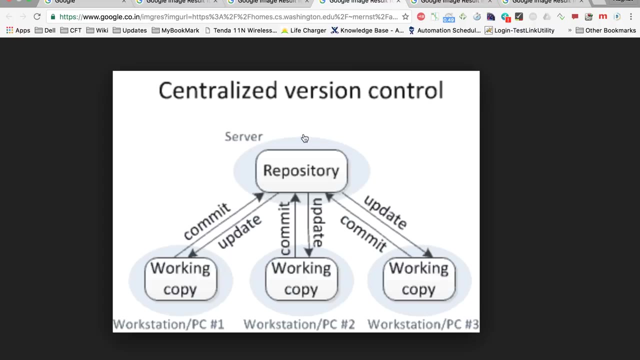 control system, And then we have a centralized version control system, And then we have a distributed version control system. Okay, now, what does this mean is let us again look at the centralized version control system. Here we will have a repository which is placed. 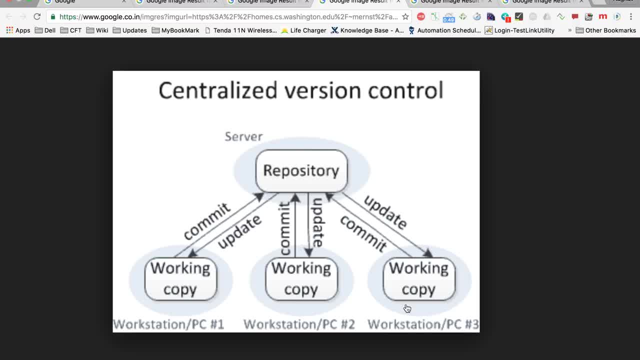 on a server and then there are different people working on that repository. So you can see this is workstation PC number one, workstation two and workstation three, And then we have all the whirlpool results and all of these guys are working on this repository. now what? 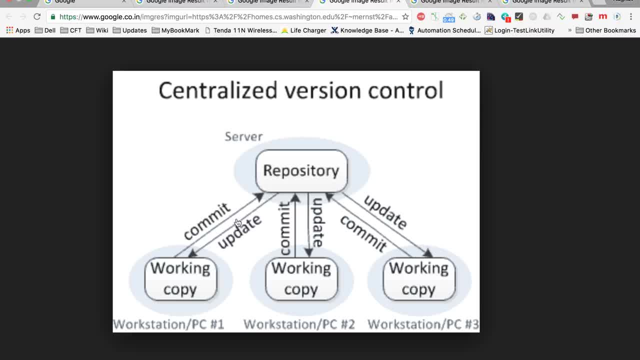 they do is they work on this repository online, make their changes committed, and so they can collaborate. Okay, but here is a major disadvantages: that this is a single repository which is replaced on a server, So if anything goes wrong here, because we have a single copy placed on the 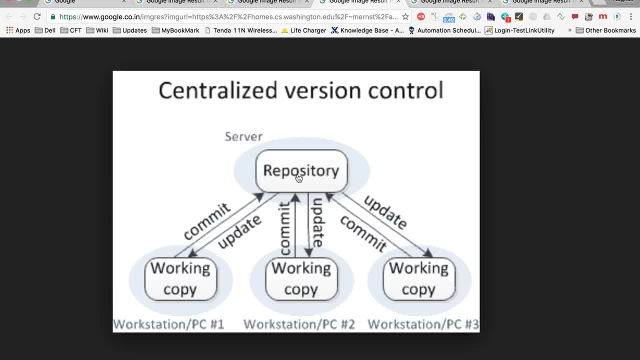 server. if anything goes wrong here, it will be difficult for us to maintain the backup and bring the repository to the normal position. also, the people who are working on this repository have to be connected always and have to be online to work on their systems because this repository is placed on. 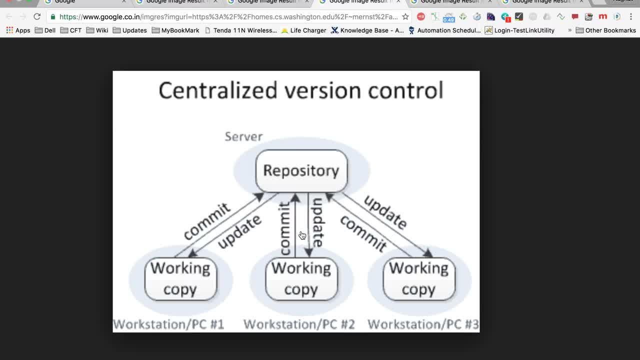 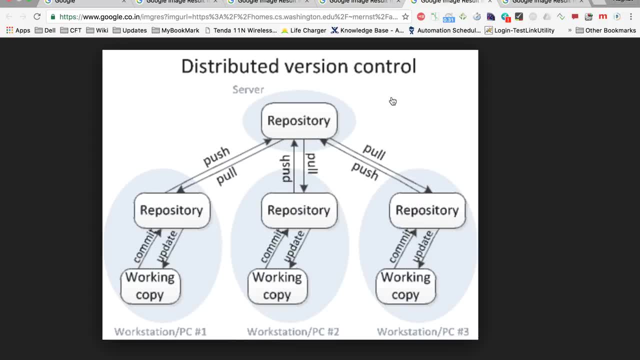 a server, so these people have to be online to collaborate. okay, so this is what a central version control system is, and then we have a distributed version control system. now, here there is a repository on the server, as we have seen in the central version control system, but every person 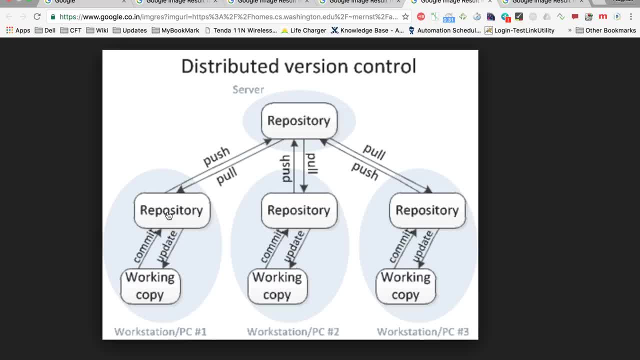 can pull and create his local repository. so you can see workstation 1 has a local repository, workstation 2 has his own copy, workstation 3 has his own copy. so one of the major advantage of distributed version control system is if anything goes wrong here on the server, we 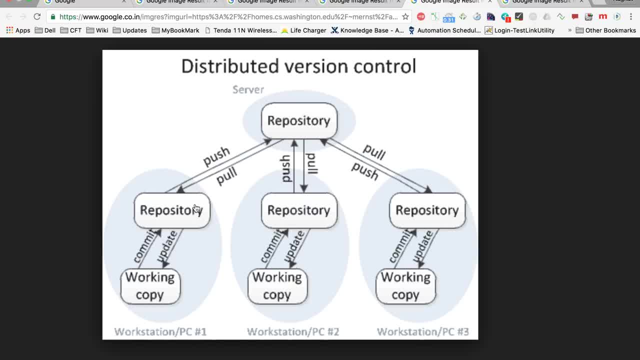 can backup the repository from any local system, because these are the complete copy of the repository. that is one major advantage. the second major advantage here is you do not do not need to be online every time. you can pull the repository, take your local copy and keep on working on it. 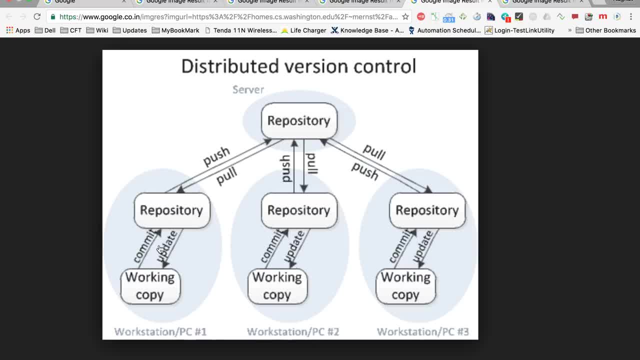 in an offline mode and you will need an internet connection only when you want to push the changes. so only when you want to push or pull you need to be connected. otherwise you can keep working offline and maintain all your work and once you are done you can push the changes. so this is the advantage of a distributed version control system. 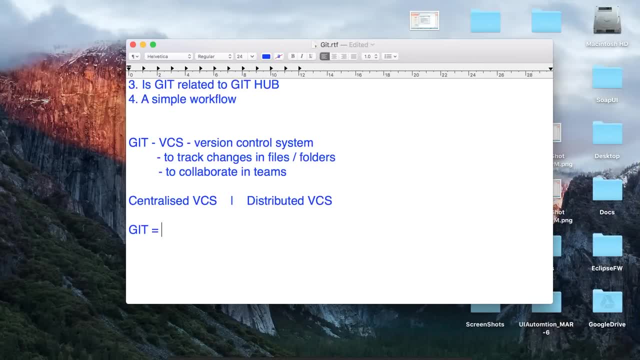 and you might have guessed by now, git is a distributed version control system. okay, and that is why git is very fast and easy to use. and you can see that the system is very fast and easy to use, famous, popular, and it is also free and open source. so i'll also write here it is. 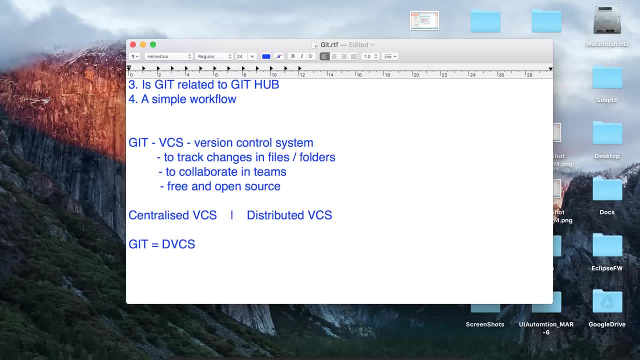 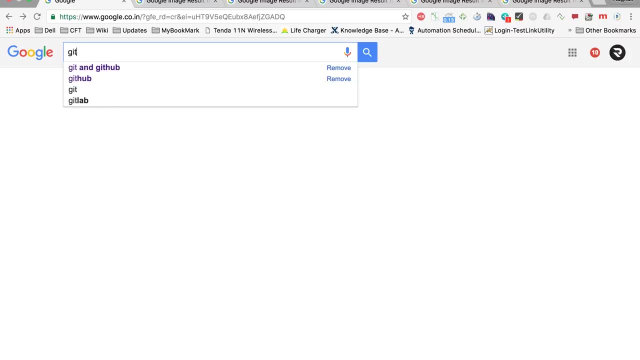 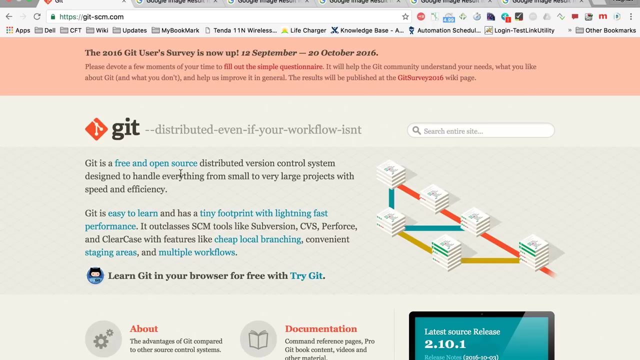 free and open source system, so a lot of people use it. okay, now let us see. let us also go to our browser and see about git. so this is the website i'm going to, git, scmcom, and here they say: git is a free and open source distributed version control system designed to handle 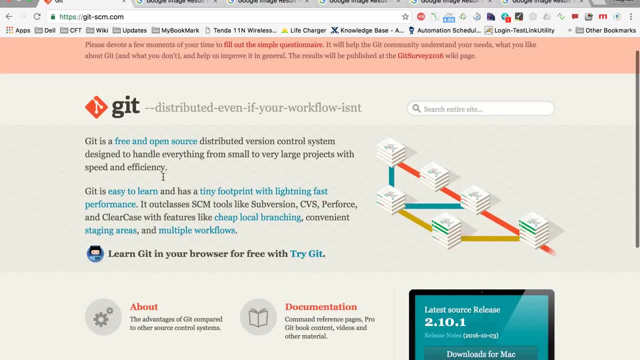 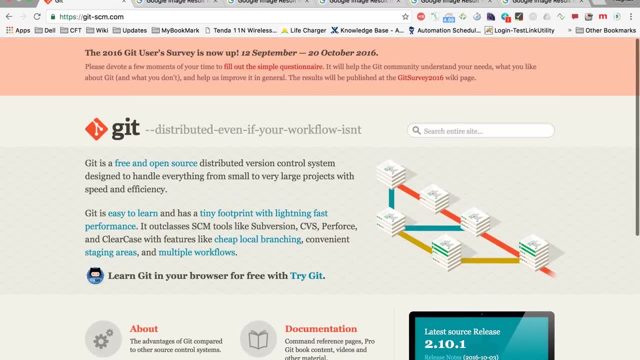 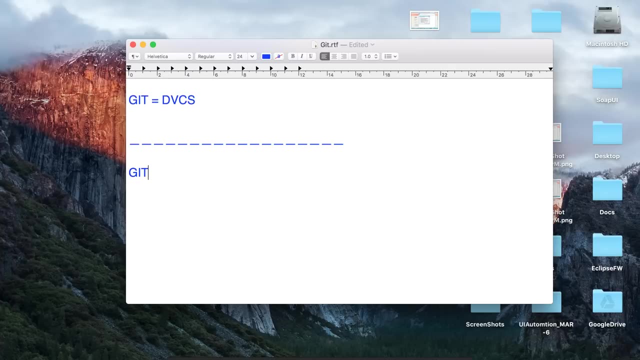 everything from small to very large projects. okay, and in the coming session we will see exactly how to download and get started with git. for now, let us go to our second topic, which is github. okay, now, github is, you can say, a website to upload your repositories online. okay, so if we go to again google and say github, 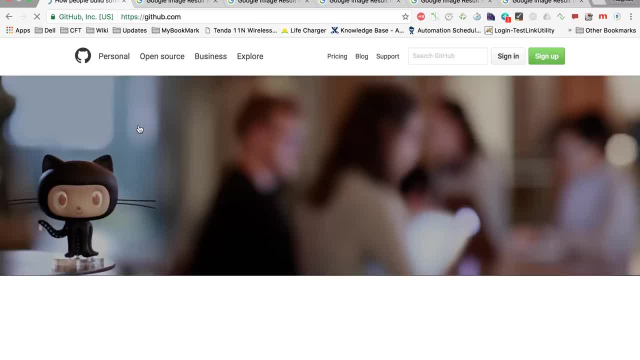 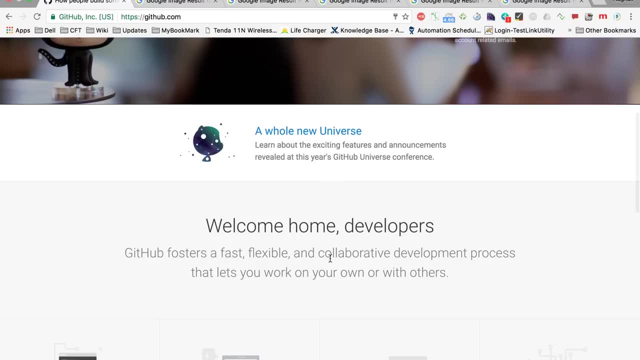 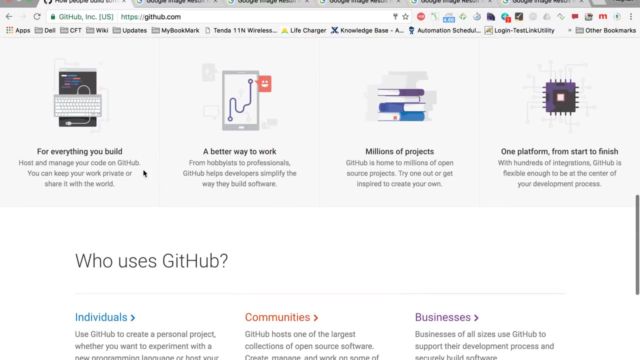 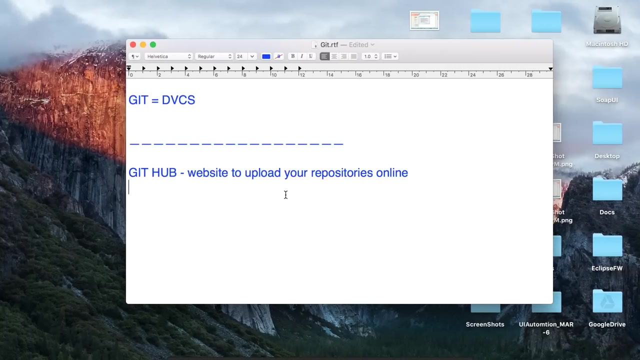 it will take you to this website of github and you can see this. github foster is a fast, flexible collaborative development process and that lets you work on your own or with others. okay, and you can use github for putting all your git repositories online, or any any repositories in that sense. okay, so in very simple words, github is a website which you 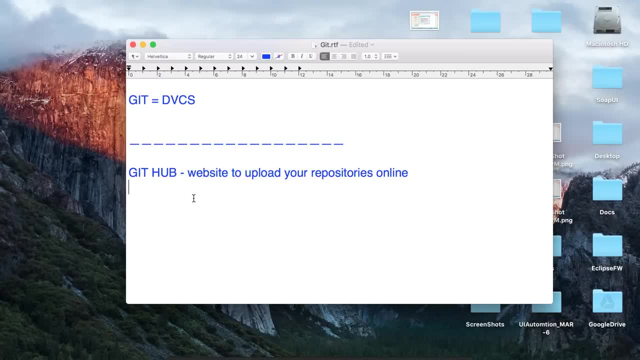 can use to upload your repositories and what are the advantages of this? why do you want to use it? it number one is it provides a backup for your repository, so your repositories are now backed up on cloud. ok, so that is a very the major advantage of using github. other thing: 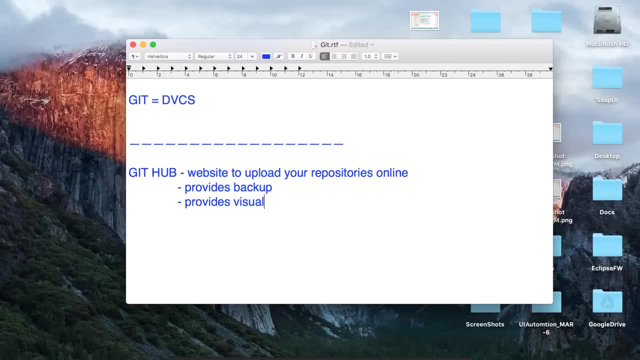 is it provides visual interface to your repositories. so when you go to, when you add your repositories on github, you can go to the github page and you can view and it provides you a very nice visual interface. ok, the other thing will be: it makes collaboration easier. so what you 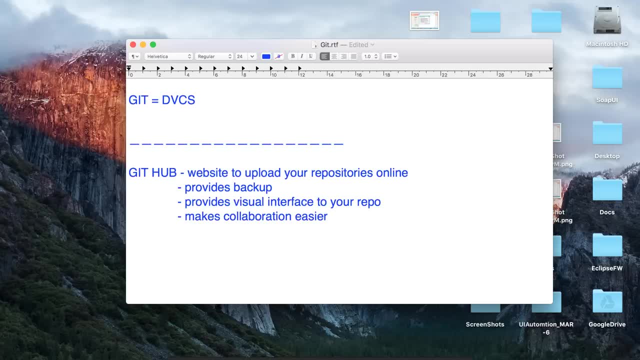 can do is you can add your repositories to github. you can make it private or public or share with some people, and it makes very easy to collaborate your repositories with other people on your team. So that is what github is. it is a website to upload your repositories online. so now 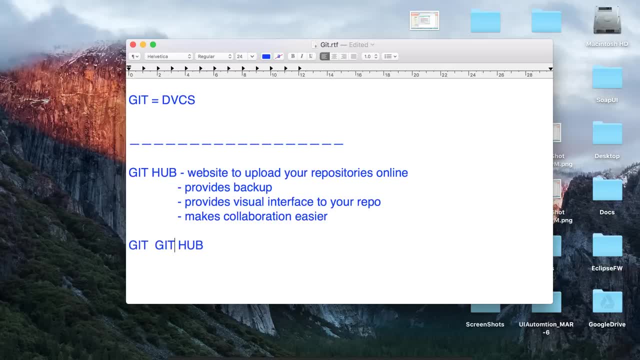 is git related to github? the answer is no. git is not equal to github. git is a version control system, whereas github is just a website where you can put your repositories. so you can use github with any version control system: it can be git or it can be some other version. 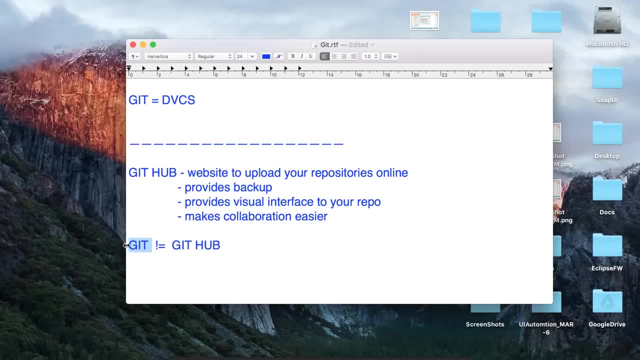 control system. In the same way, you can use git with any online repository management system. it can be github, it can be bitbucket or anything else. so you can use git with github or you can use git with some other online management repository system. git is not related to github, although 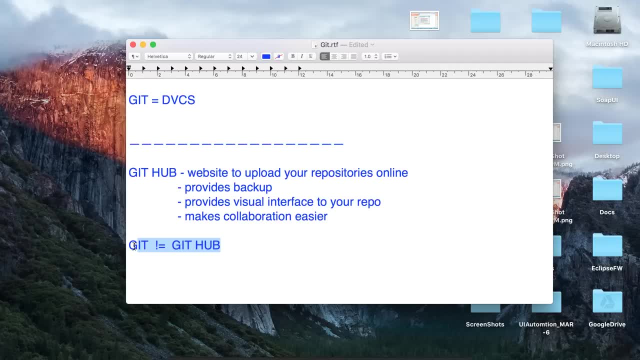 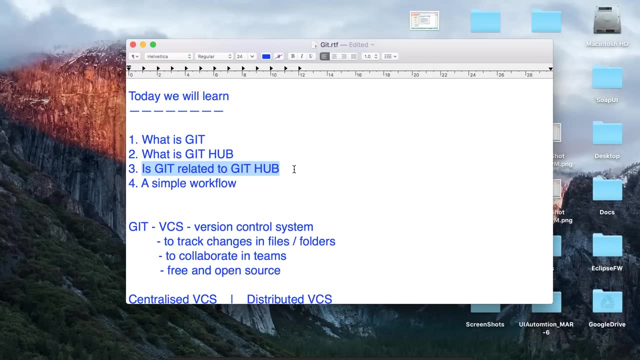 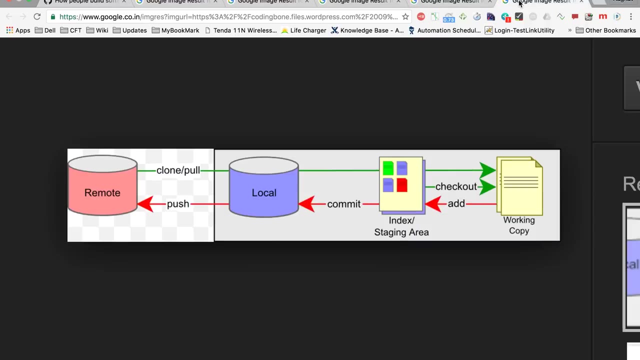 most of the projects use git and github together, but technically they are not related. ok, so this is the. there is no relation between git and github. they are two different things. okay, now let us look at a very simple workflow of git and let us look at this diagram. so uh, 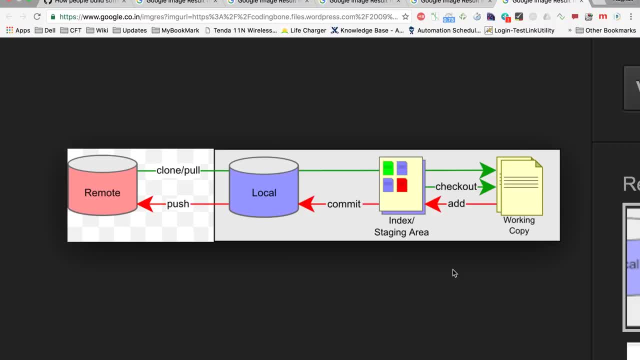 when we actually start using git in our next session. what we are going to do and what the actual workflow looks like is: this is a remote repository and this is our local system. let us say our repository is put on a server, it is placed on a server.